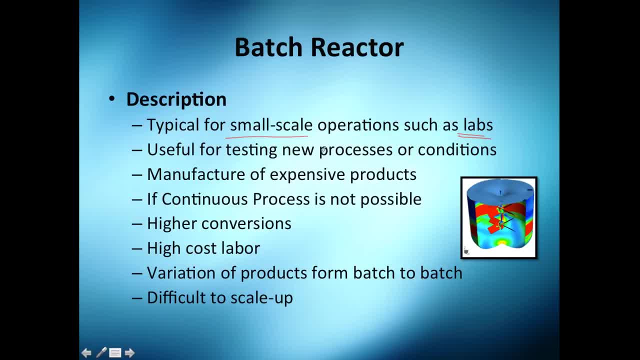 So why not just check it first in the batch reactor? If it works, then we try to scale it up. Now the manufacture of these products is expensive, so that's not good. Because of the same, each batch costs a lot. 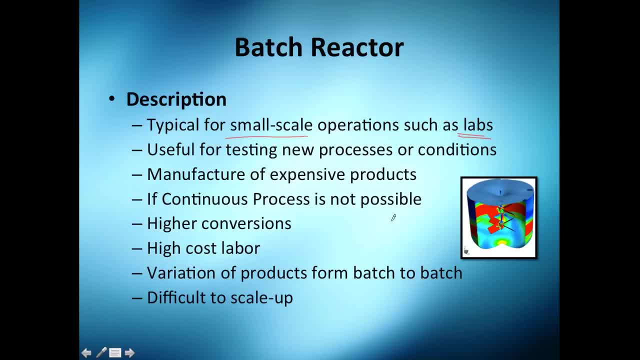 If you cannot do a continuous process, which is normally the case for many small industries, you cannot have someone operating the plant all day, all night, all year long. So if you cannot do that, the recommended reactor will be the batch reactor. 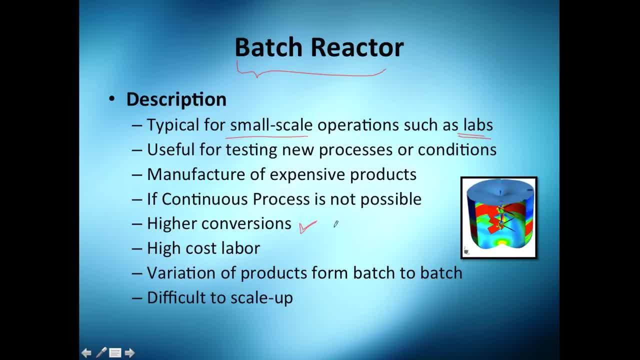 The good thing is that you can get high reactions because it's so into the reactor. You give the time needed to the reactor, so every batch gets relatively high conversions. High-cost labor, of course, because you need someone cleaning and operating and all that. 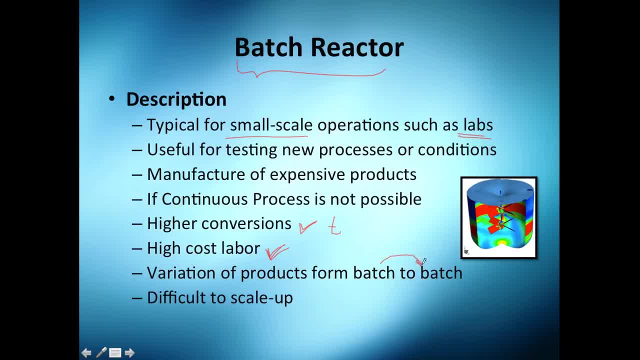 And the variation of products from batch to batch is a problem. maybe The thing here is that from batch to batch every batch is maybe unique. So you got good properties, bad properties, different properties in all the batches. It's sometimes difficult to scale up because maybe in lab or in a pilot 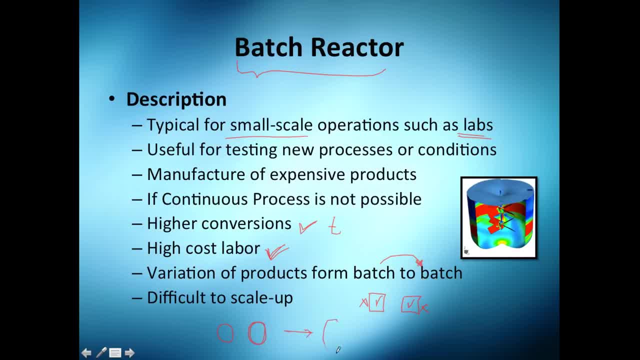 a small- let's say medium- scale is okay, But when you go huge, you got different phenomena that you weren't aware of. For example, mixing. You mix a huge amount of material. It's difficult to mix it, But in the lab it's so easy to mix a beaker or a cup of water. 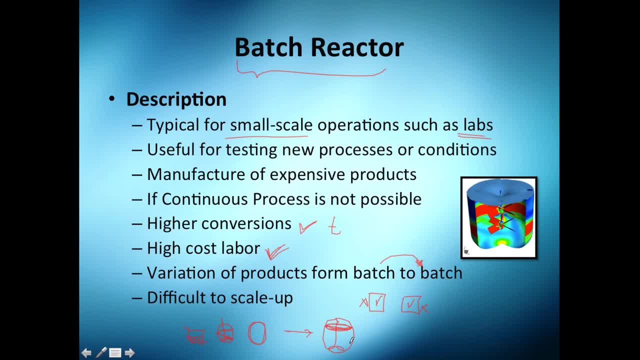 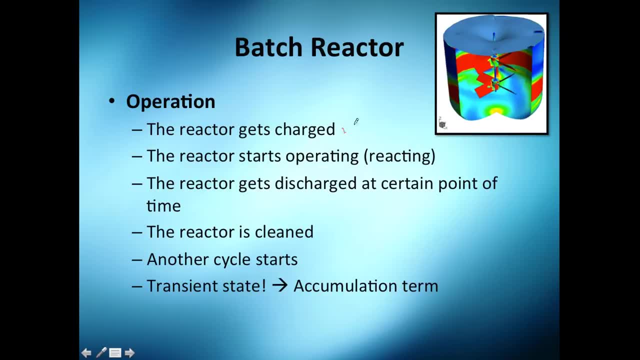 It's so easy to mix it, But when you're talking about a huge tank here, well, it's not the same. Now something about the operation of the batch. The reactor gets charged, So you got this empty reactor. Of course, you need to be sure it's clean. 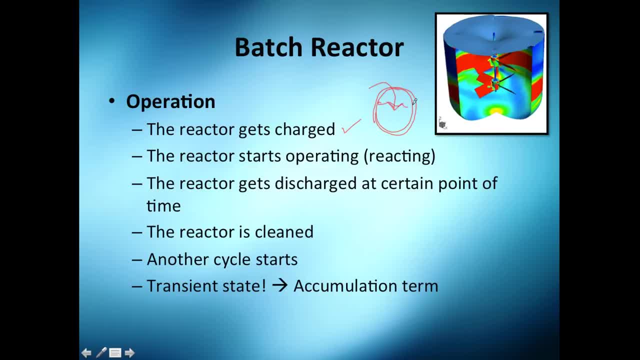 Then you charge it, The reactor is turned on, So all the temperature spreads, The pressure levels are controlled. You start reacting, reacting, reacting. That's called the operation. Then you stop it. You discharge the batch at a certain point of time. 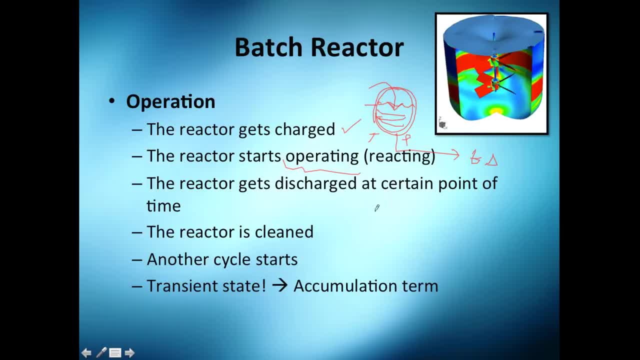 You give it a certain time, It's very important. And then, well, you got this- let's say- dirty reactor, You clean it And you start the cycle again. So that was batch number one. What would you do? 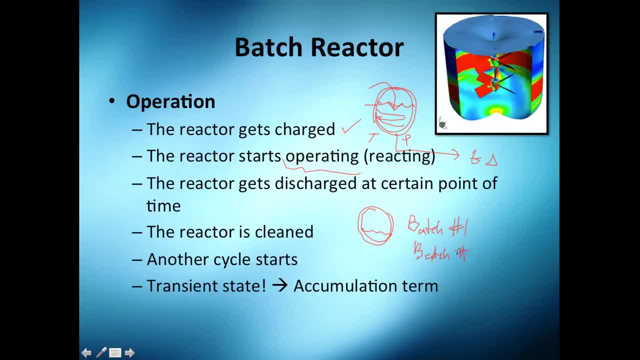 You will do the same thing and you will get batch number two And you will do this until you get to the final amount of required amount. The thing here is very important to let you know that this is trenching state, So there will be an accumulation term on the equation. 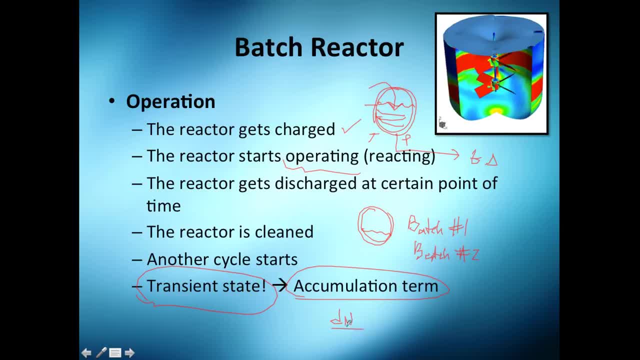 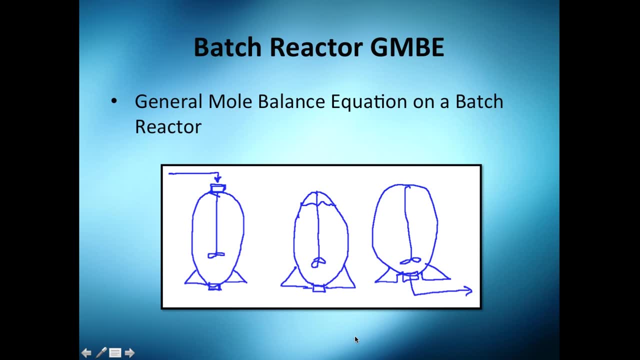 What does that mean? You will have a derivative of something, especially mols, with respect of time. So concentrations, mols, products are changing with time. Now let's apply the general mol balance equation. So, general mol balance equation: As I told you, there's a charge. 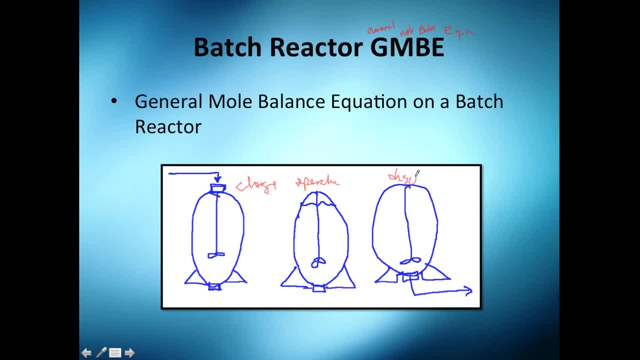 There's the operation part And there's a discharge. The thing here is that many students always think that we are analyzing this and this and this part, And the actual truth is we are only analyzing this part. There's no reaction here. There's no reaction here. 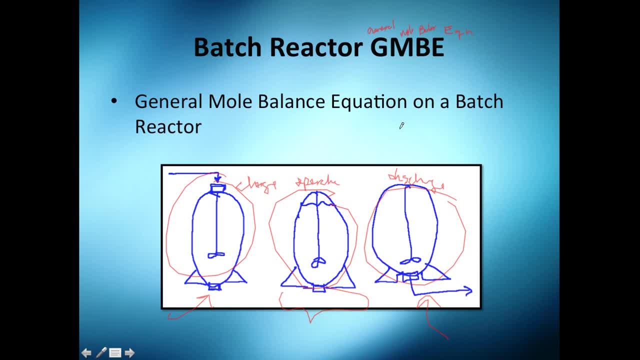 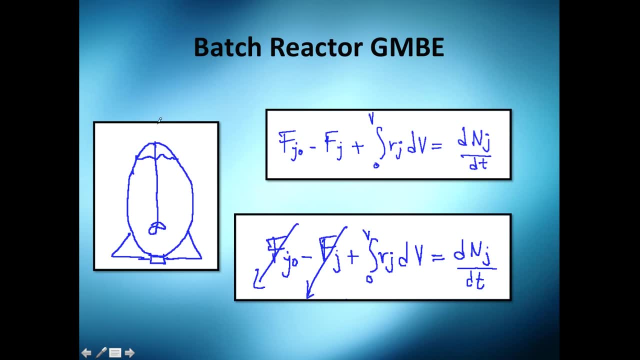 So why do we apply a molar balance equation to things that are not reacting? It doesn't make sense. So we're going to analyze only this, And it's very important because when I get this equation, the master equation, I got inlet. 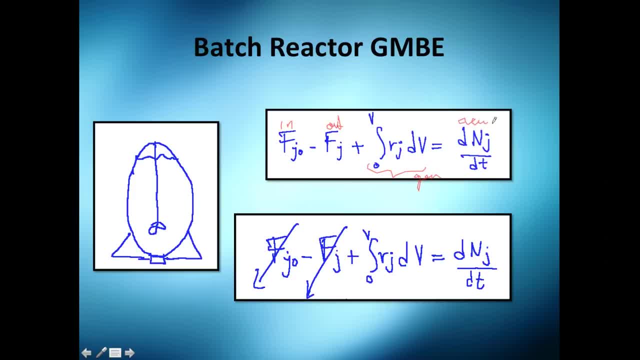 I got outlet, I got generation And I got the accumulation term. And many students tell me: of course you got an inlet. You got an inlet because you are feeding the batch reactor And of course you got an outlet because you are discharging the reactor. 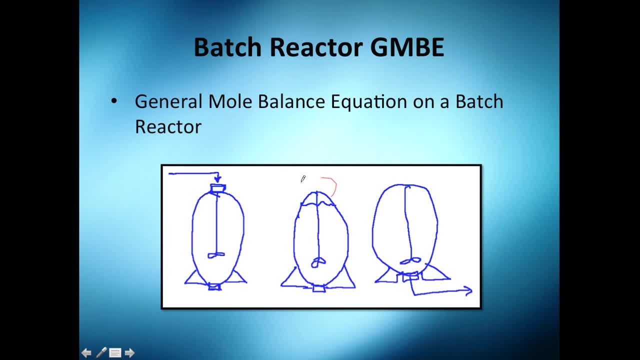 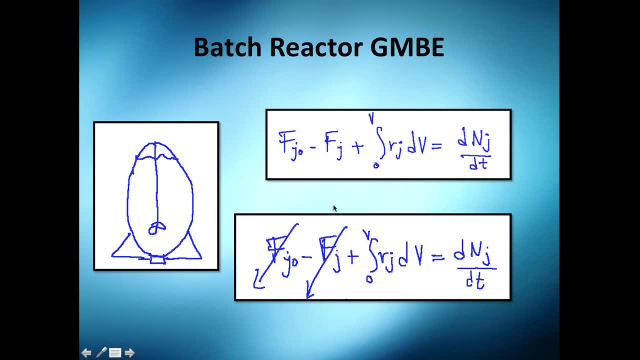 But as I told you before, guys, we are analyzing only this part in which we are reacting. We are not analyzing this discharge process, nor this charging process. So what happens? We have no inlet, no outlet. As you can see, it's already everything inside. 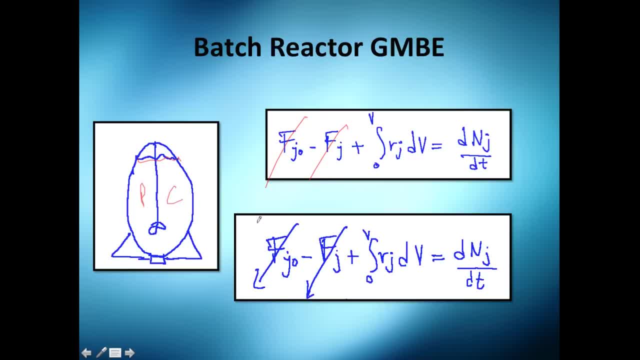 Generation. of course we have generation. We have production and consumption of materials. Actually, we are producing material and we are consuming reactants. So please never take out this in any reactor. The point of a reactor is having a reaction. So if you take away that or if you take away this, well, it doesn't make that much sense. 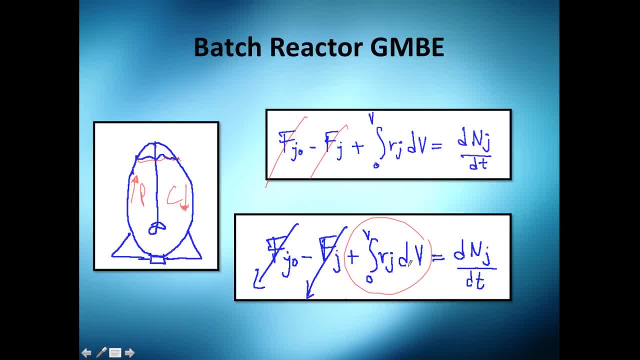 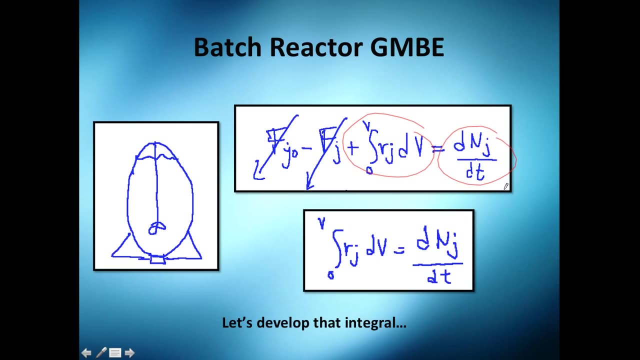 that you are doing a reactor balance in a reactor when there is no chemical reaction And the accumulation term. yes, we are changing material with respect of time. So we get This here, This equation. This cannot be taken away and this cannot be taken away. 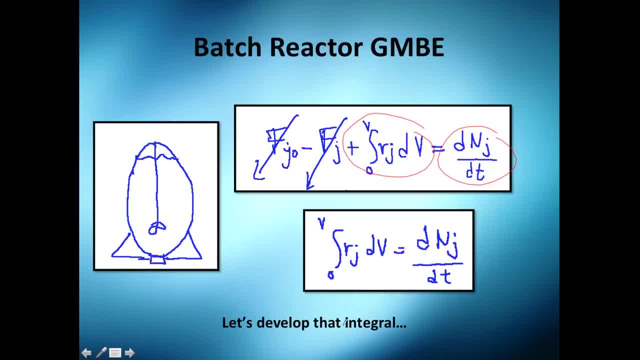 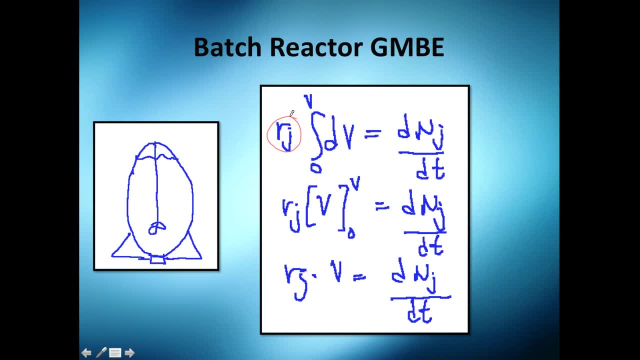 So actually you can end it here, but I'm going to develop that integral. We got this here. I take out this because this does not depend on the volume. Let's say it's uniform, It's perfectly mixed. So in this point and in this point and in this point, all the rate of reactions are the same. 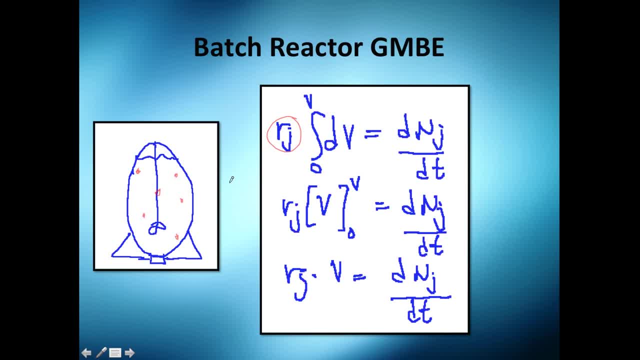 Which is kind of ideal. yes, I know, But we are doing this Because it's our first molar balance in a batch reactor, So we want to call it ideal. So we take it away from the integral. Then what do we do? 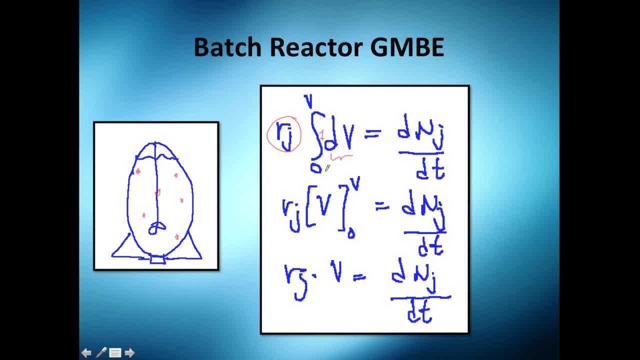 As you can see, there is a one, So the integral of one is volume here And we need to evaluate it in zero and volume, Which will be essentially B minus zero, which is B. So I got this here, Which is my rate of reaction of J times volume. 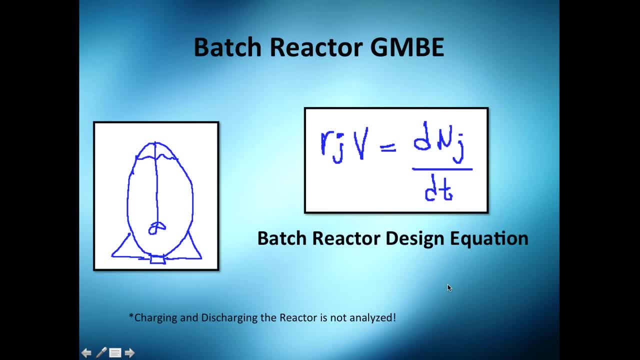 And the accumulation term. I just drop it here. Good, So this is my batch reactor design equation. Please, if you don't understood what I just did, check it again, Because it's so beautiful how the rate of reaction times, the volume, will give you the amount of this and this. 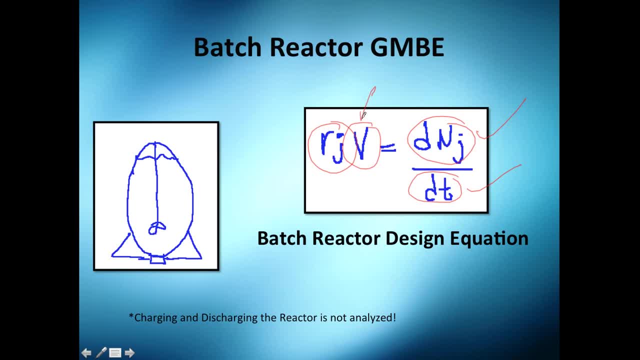 And, as you can see, we got either time, moles, volume and rate of reaction. How do you get this rate of reaction? If you have lab experiments in literature, they will give it to you Or, worst case scenario, you do it by yourself with experiments.